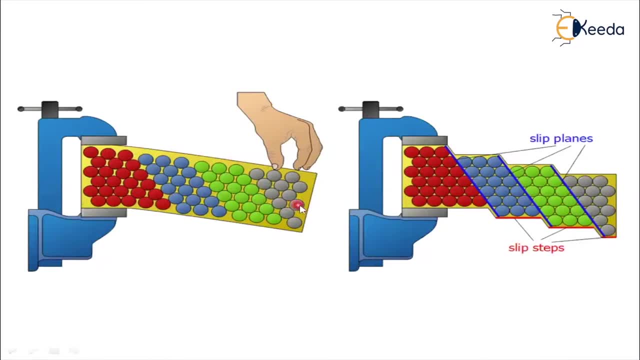 It can be deformed to a length many times to its original shape, but upon release it returns to its original shape and size. For this reason, an object undergoes elastic deformation Before plastic deformation is observed. Now, what do you mean by plastic deformation here? 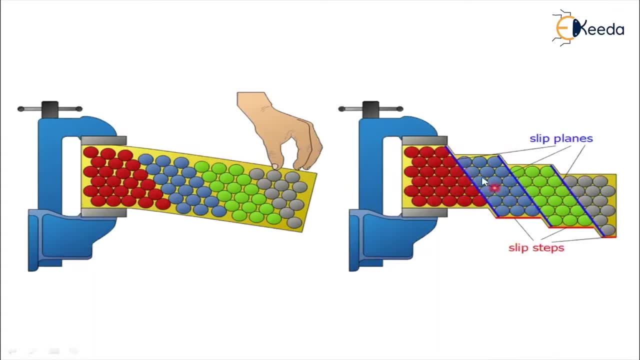 Plastic deformation occurs when the bonds between atoms are broken. You can observe here: Suppose, assume these are some number of atoms. These are another number of atoms. Between these two atoms the bonds are broken. here, like this, A new one is formed. 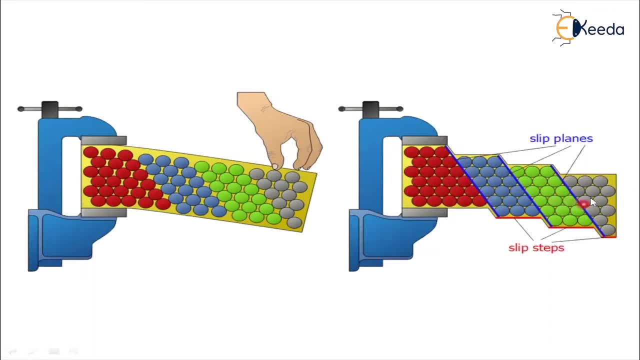 Making reversal to the original shape is highly impossible. But here, even though the atoms are different, when you apply load, after removal of the load, again these atoms again formed into the same shape And again they get back to the original form. 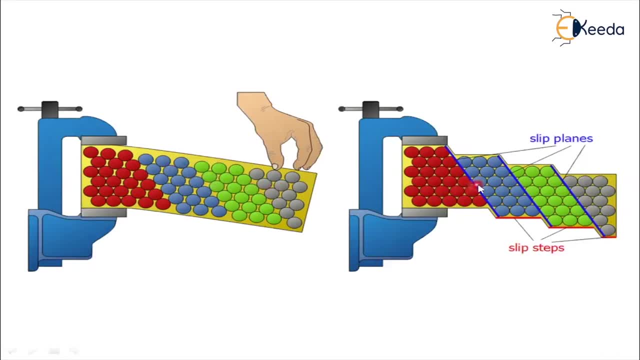 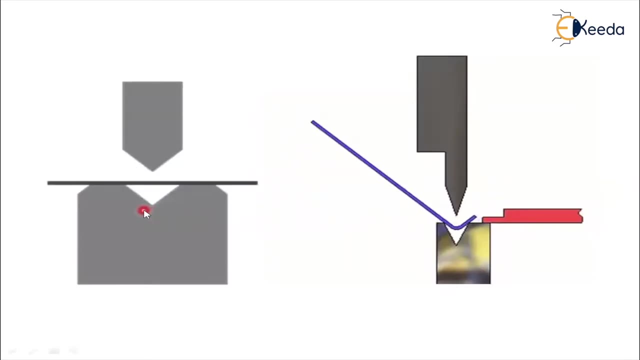 That is the main difference between elastic and plastic deformation Here. so many slip planes may be observed in plastic deformation. This is called as permanent deformation. We can observe the plastic deformation with some more images like this. These images show how the material undergoes plastic deformation when the load is applied. 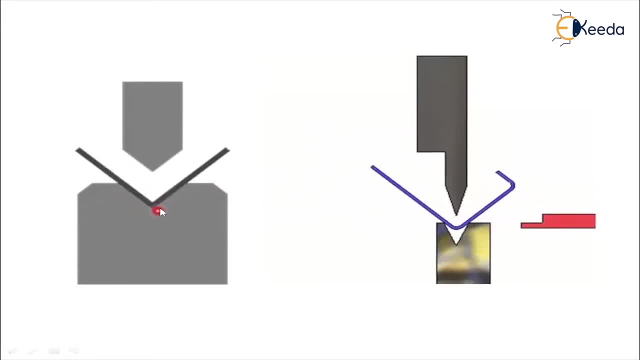 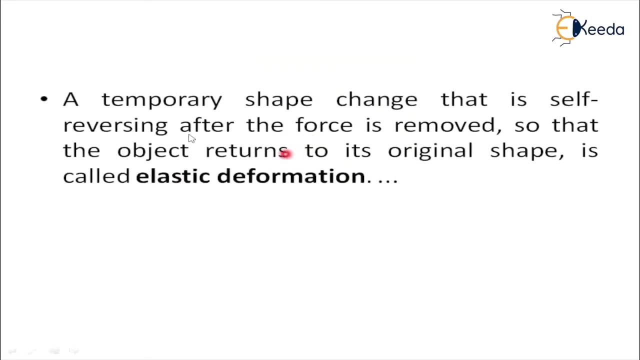 The plastic deformation. we already said that it means once it is deformed, it will not regain its original shape. Let us discuss the definitions. What is the definition of elastic deformation? Let me explain this: A temporary shape change. Here the main word in elastic deformation is a temporary shape change, that itself reversing after the force is removed. 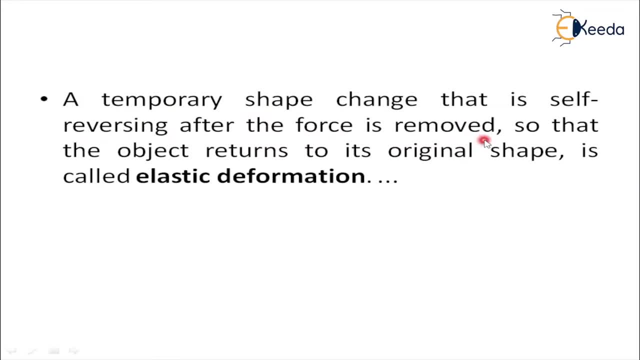 That means once the force is removed, it will get back to the original form, So that the object returns to its original shape. It is called as elastic deformation. Now, what is plastic deformation definition? Here is the definition: When the stress is sufficient. this word is important. 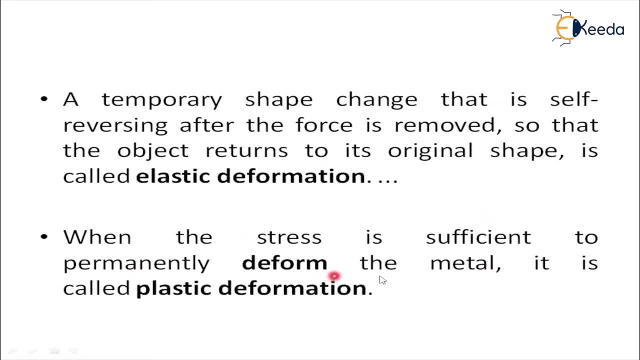 When the stress is sufficient to permanently deform the metal. So that means if the stress is not sufficient, then we cannot say that the material undergone plastic deformation. This sufficient word is very, very important in deforming the material or any metal. Suppose if the material undergone, or if you apply the less energy or less stress on the material, then we can say that the material undergone elastic deformation only. 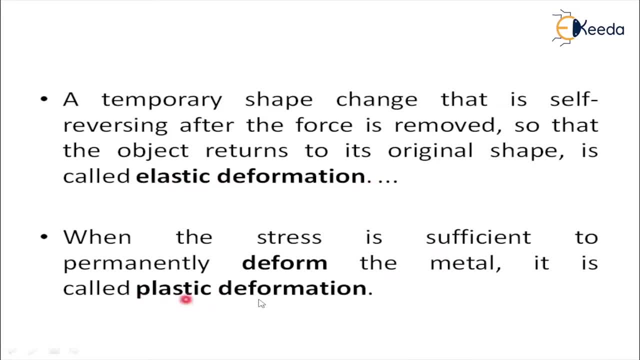 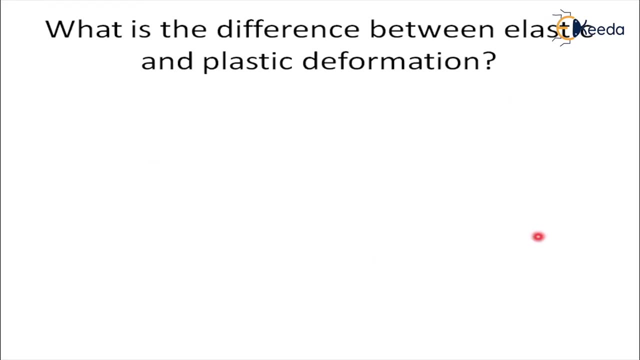 Sometimes we can clearly see the temporary plastic deformation Means only half of the energy is utilized by the material. So we will see some more features regarding elastic and plastic deformation. First of all, try to understand the difference between elastic and plastic deformation. Here the main point is: elastic or plastic depends on the type of the substance. 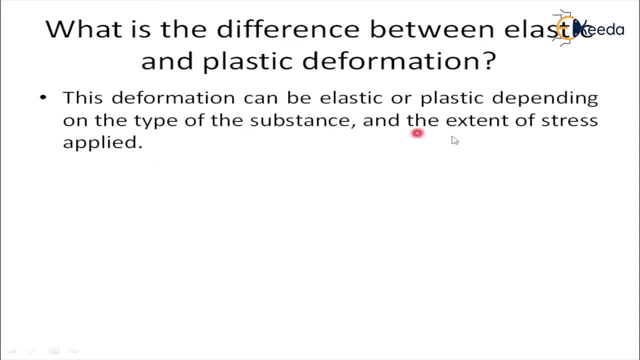 What do you mean by type of the substance here And the extent of stress applied, How much stress applied, How much stress is applied And what is the substance type Means if the substance is having brittle nature. one type of graph you can see here: 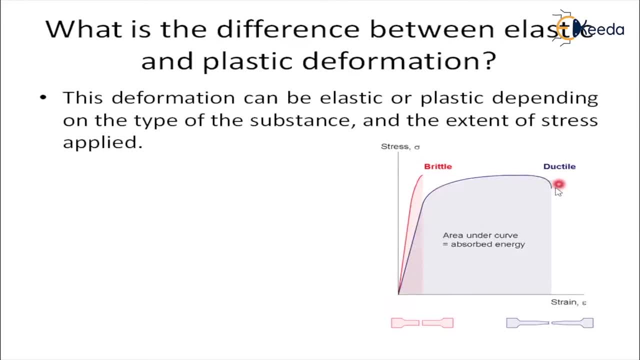 If the substance is ductile in nature, you are observing another graph. So that means elastic or plastic. deformation is completely depends on the nature of the material. So that means type of the substance. Steel shows one type of property and glass will show another type of property. 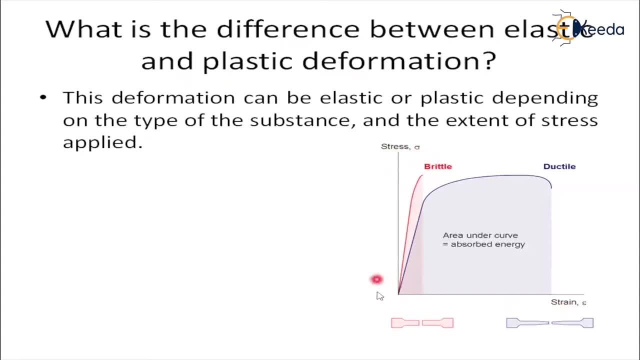 So that means stress is directly proportional to strain, even though this graph is showing the stress is directly proportional to strain. But for all the material the graph is not same. You can observe the material here. This is the necking area When the tensile load is applied. 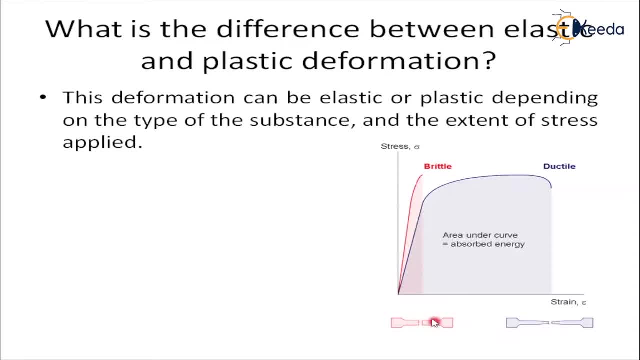 How the deformation is happened. For brittle material, For ductile material, You can observe a clear difference between the brittle material and ductile material. In brittle material, without having any deformation, the break is observed, But here the deformation, here the elongation is observed. here 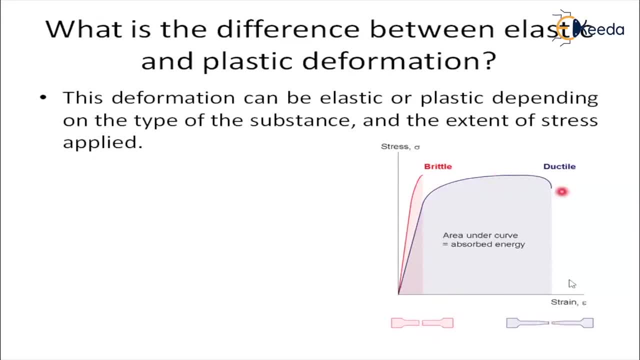 After some elongation at last, the break is observed. in the case of ductile material, The main difference between elastic and plastic deformation is that the elastic deformation is reversible And the plastic deformation is irreversible. That is the main difference here. Now we will observe some more. 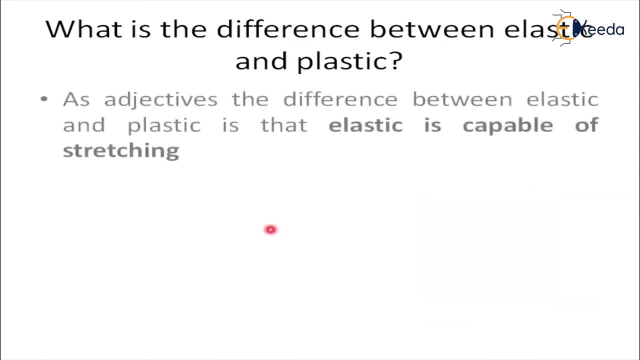 We will observe some more salient features. Elastic is capable of stretching- The name itself is represented as elastic- is capable of stretching, Particularly capable of stretching so as to return to an original shape or size when force is released, While plastic is capable of being molded. 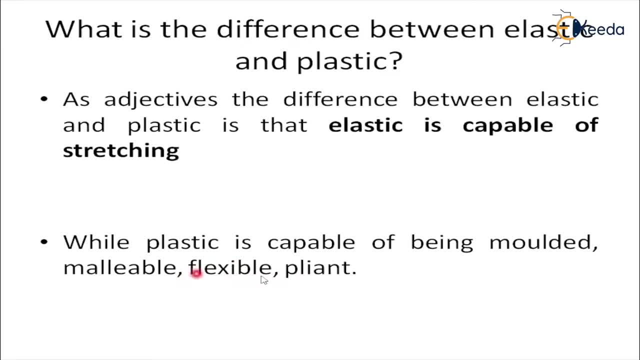 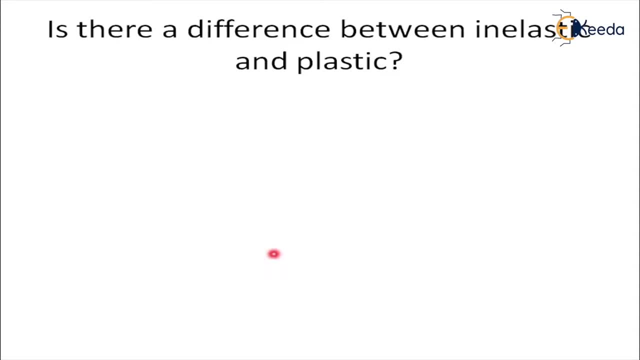 Flexible and flying. So these are the main features of plastic deformation or plastic. Let us discuss with some more images, And first of all Observe the two words here: Inelastic and plastic Elasto plastic. What do you mean by elasto plastic here? 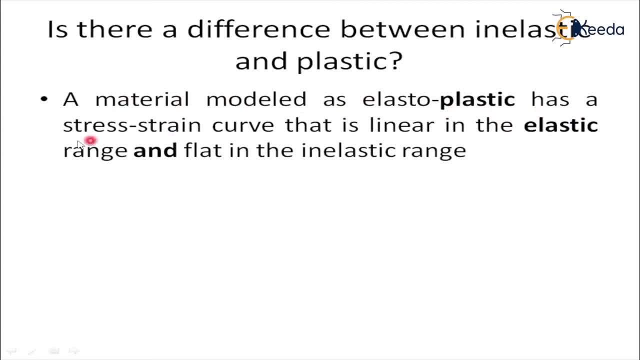 A material modeled as elasto plastic. Elasto plastic has a stress strain curve that is linear in the elastic range And flat in the inelastic range. Inelastic means it is nothing but a plastic range. here You can observe these two here. 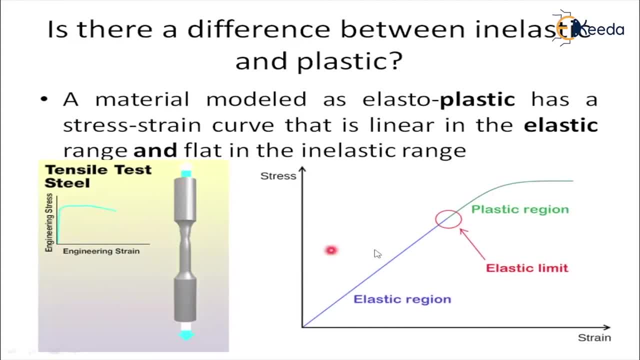 Try to identify the difference between these two figures. Here you are seeing one stress versus strain graph. Here you are observing another graph: Stress versus strain graph. Here the animation of the specimen. The specimen undergone is the ductile specimen. If it is a steel, it is a ductile in nature. 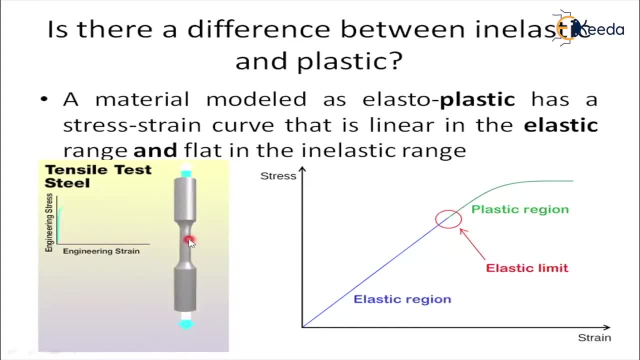 The property is ductile, So that means first of all it has to elongate. After that only the break may be observed here, Up to some extent. if you observe the graph, Stress is directly proportional to strain. Up to some extent. after that the plastic region may be observed here. 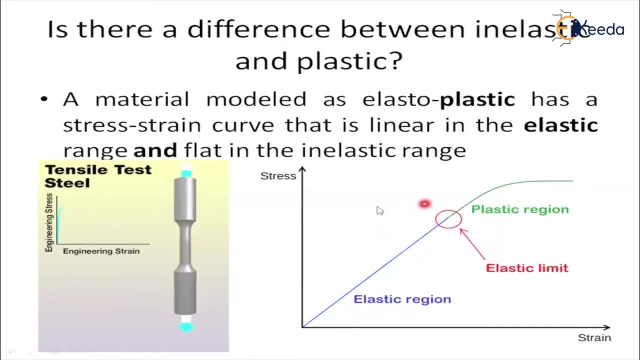 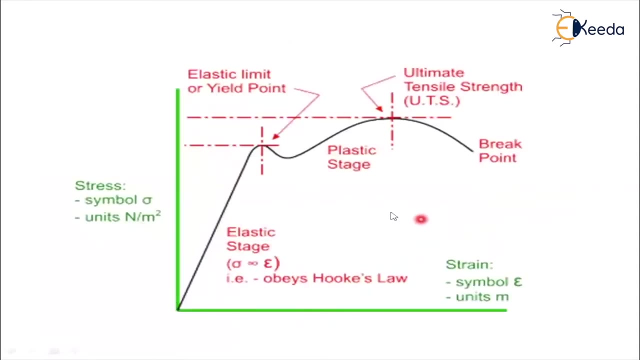 Here we are observing. stress is directly proportional to strain, Only up to some extent only. But after that plastic region starts Means, once stress reaches to its point, The material will not get its original shape. We will observe one more figure here. This is the common graph for so many number of materials. 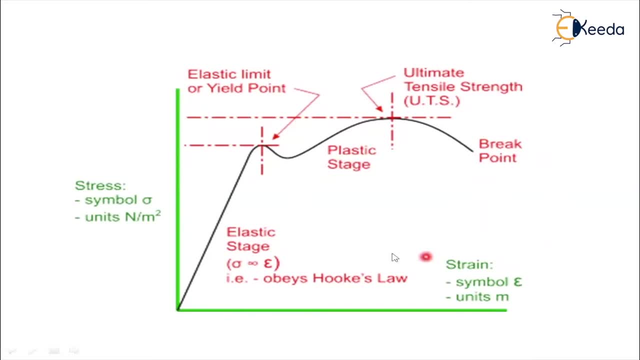 But it is not same for all the materials. We can observe the straight line up to some extent, And this is called as. stress is directly proportional to strain. This is called as yield point. How much elongation may be observed Depends on that. only we can clearly say: 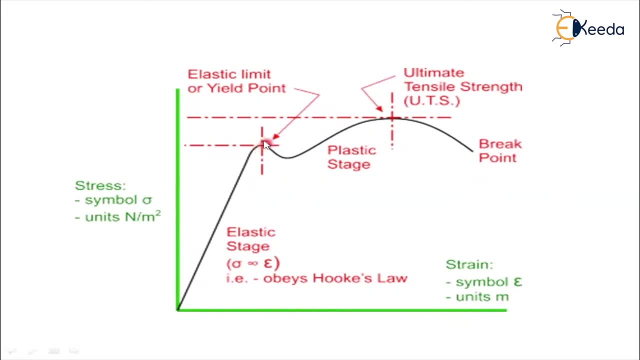 How much elastic deformation for a material. After this, this is the plastic region And after this we cannot apply the stress. This is the ultimate tensile stress. Then this is the break point here. This is the graph, Common graph for so many number of materials. 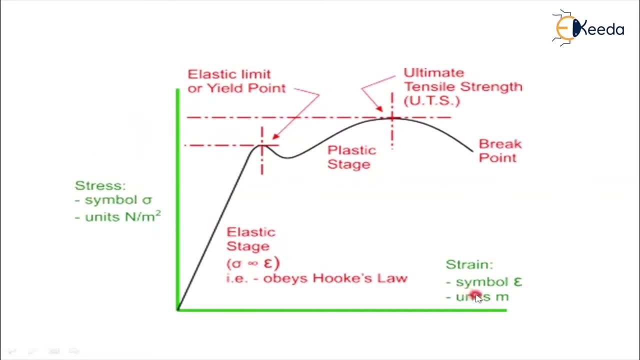 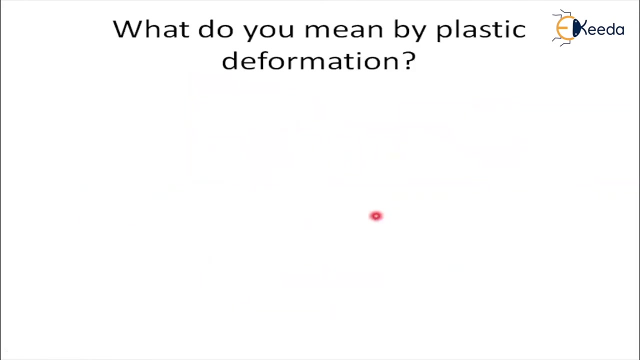 For stress versus strain. here And in this graph We can observe the difference between elastic stage and plastic stage. Here the main point of plastic deformation is- We can see the sentence here- The plastic deformation is a permanent distortion. This is the main word in plastic deformation. 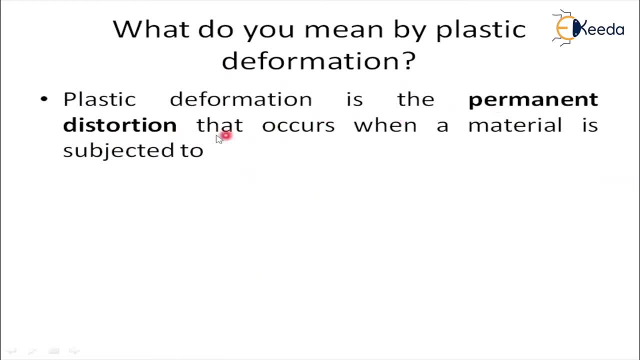 Elastic is only a temporary deformation or distortion, But the plastic deformation is The permanent distortion That occurs when a material is subjected to- First point is tensile And compressive And bending or torsion stresses That exceed its yield strength. 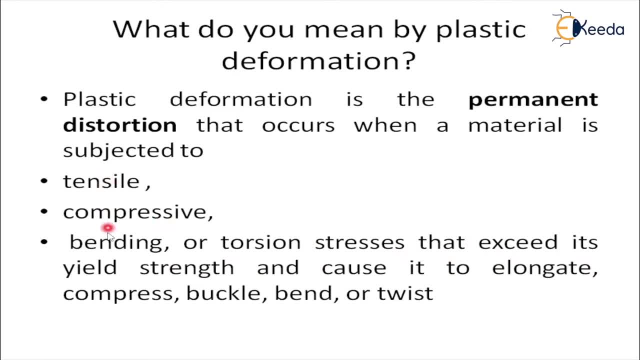 This point is important. Suppose if these stresses- Tensile, compressive, bending or torsion stresses- Exceeds its yield strength, Then only it cause to elongate, Compress, buckle, bend or twist Whatever. So all these may happen.